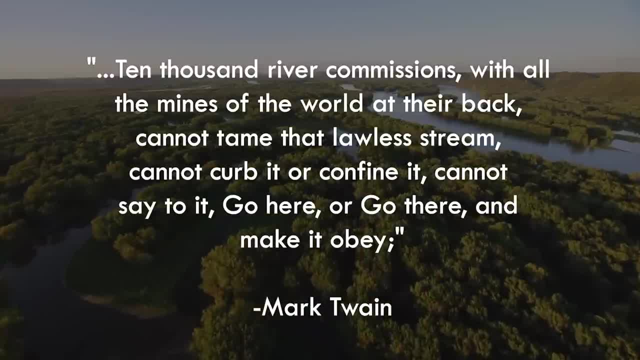 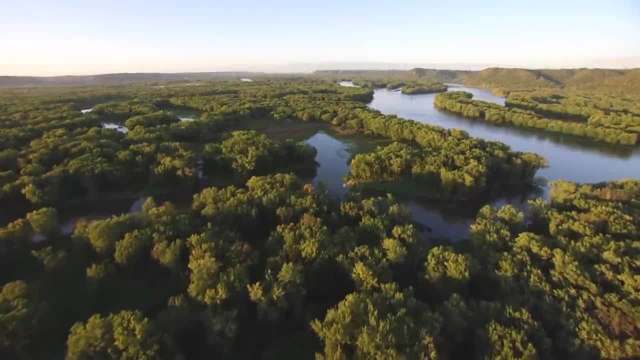 with all the minds of the world at their back, cannot tame that lawless stream, cannot curb it or confine it, cannot say to it go here or go there and make it obey. And engineers have spent the better part of the last 140 years trying to prove him wrong. In my previous video on rivers, 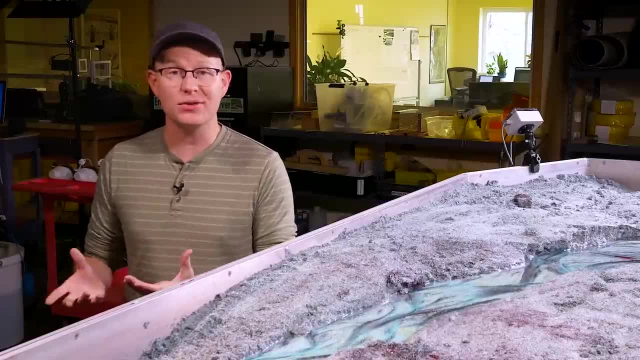 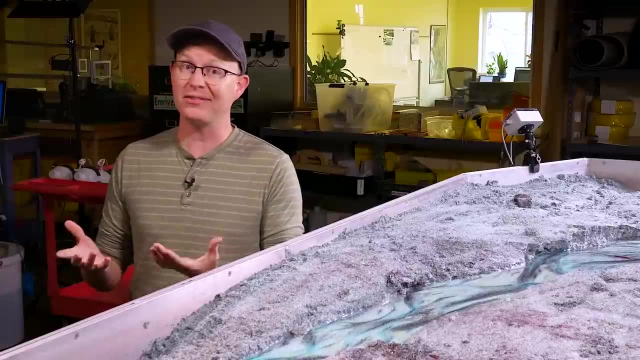 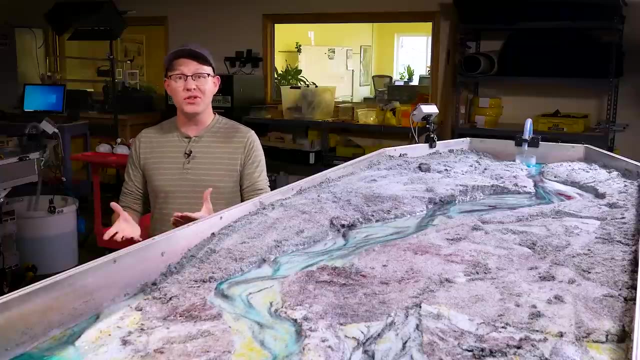 we talked about the natural processes that cause them to shift and meander over time. Now I want to show you some examples of where humans try to control Mother Nature's rivers and why those attempts often fail or at least cause some unanticipated consequences. We've teamed up with MRiver, maker of these awesome stream tables. 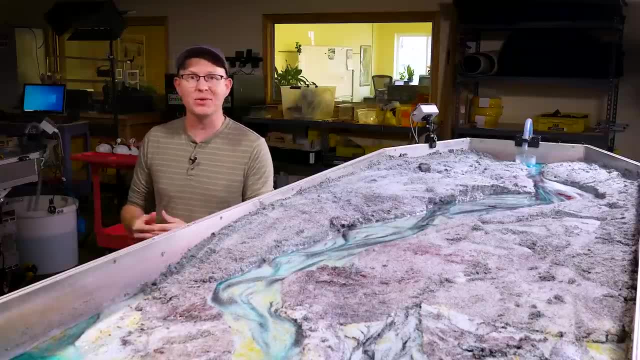 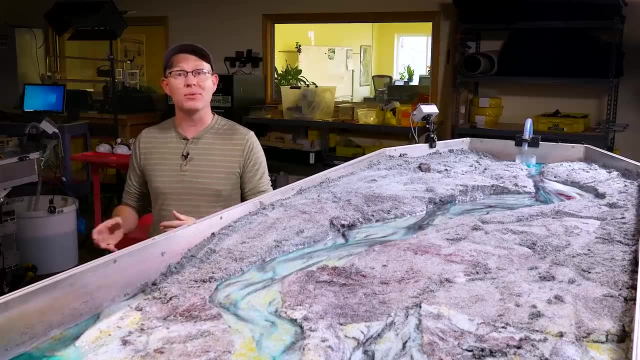 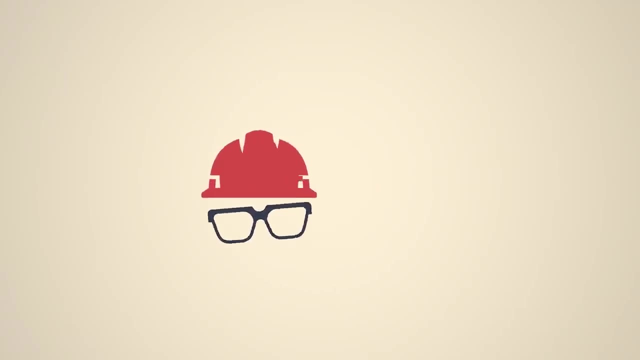 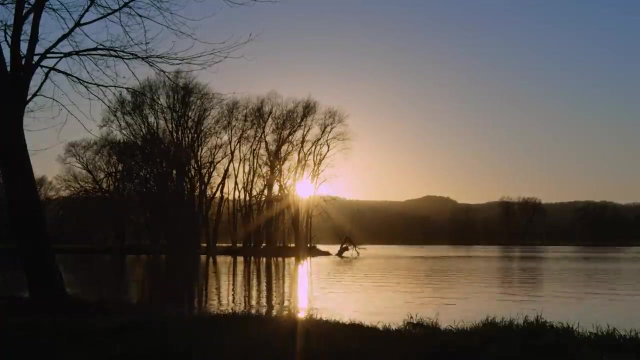 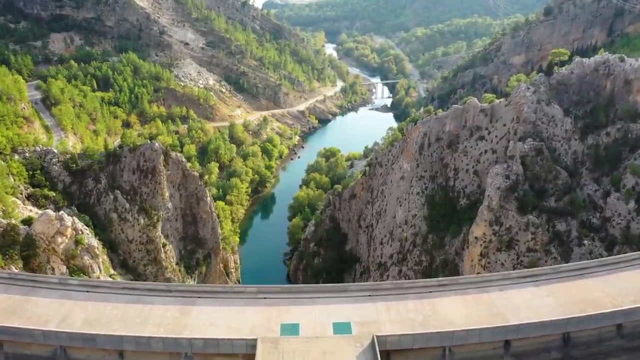 to show you how this works in real life, and we're here on location at their headquarters. I'm Grady, and this is Practical Engineering. On today's episode, we're talking about the intersection between engineering and rivers. One of the most disruptive things that humans do to rivers is build dams across them. 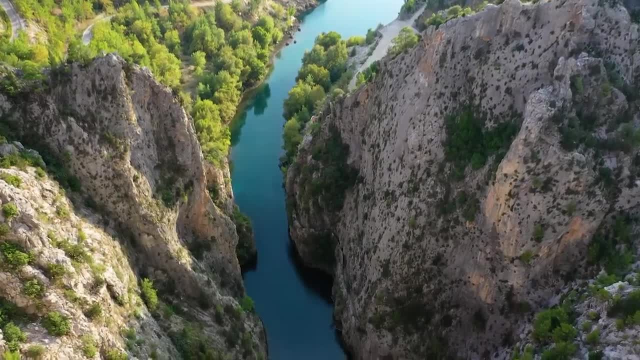 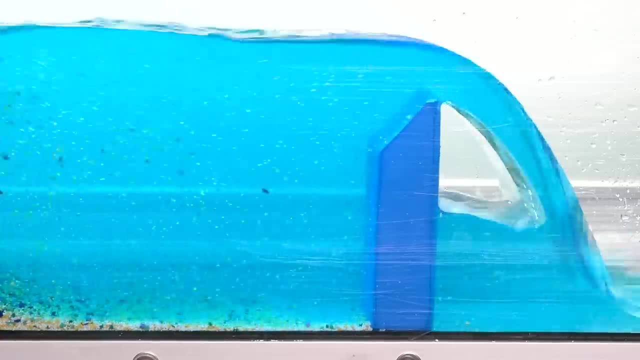 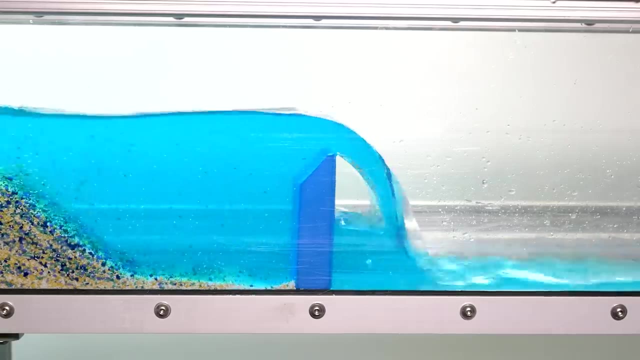 creating reservoirs that can be kept empty in anticipation of a flood or be used to store water for irrigation and municipal supplies. But rivers don't just move water. they move sediment as well. And just like an impoundment across a river stores water, it also becomes a reservoir for the silt. 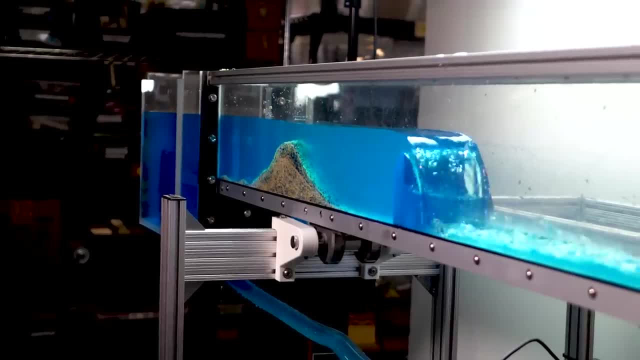 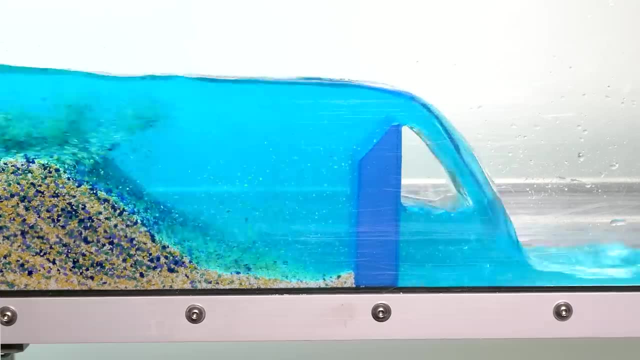 sand and gravel that a river carries along. That's pretty easy to see in this flume model of a dam. Fast-flowing water can carry more sediment suspended in it than slow water. The flow of water rapidly slows as it enters the pool, allowing sediment to fall out of suspension. 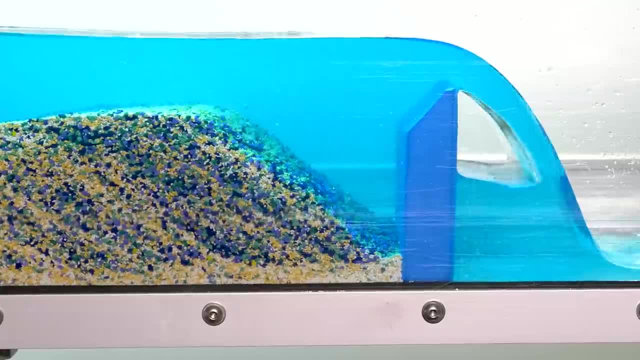 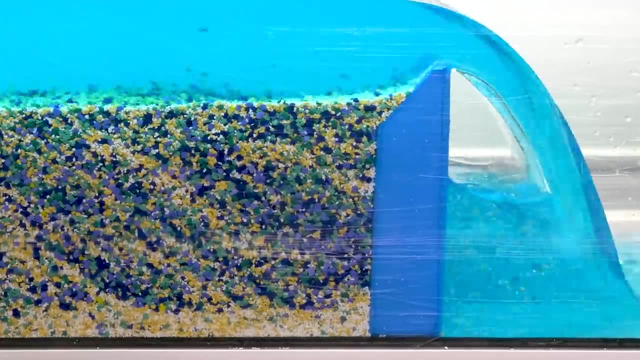 Over time, the sediment in a reservoir builds and builds. This causes some major issues. First, the reservoir loses capacity over time as it fills up with silt and sand, making it less useful. Next, water leaving on the other side of the dam, whether through a spillway or out of the works. 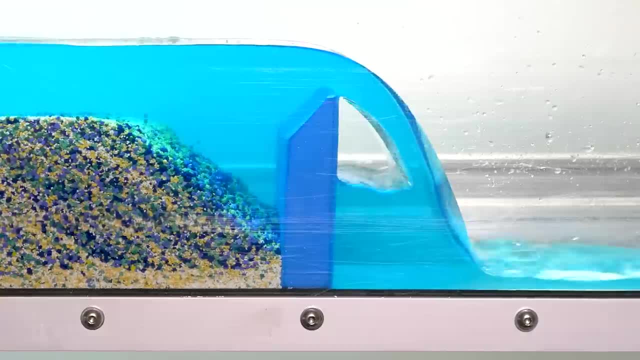 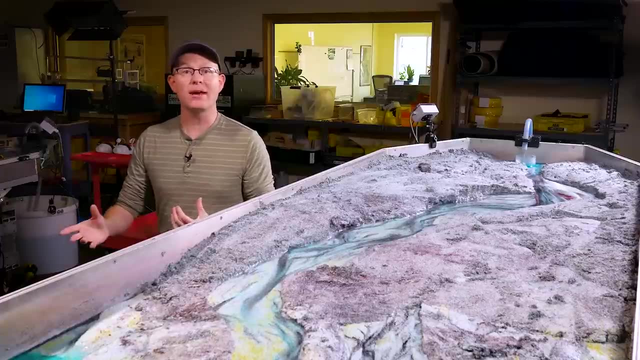 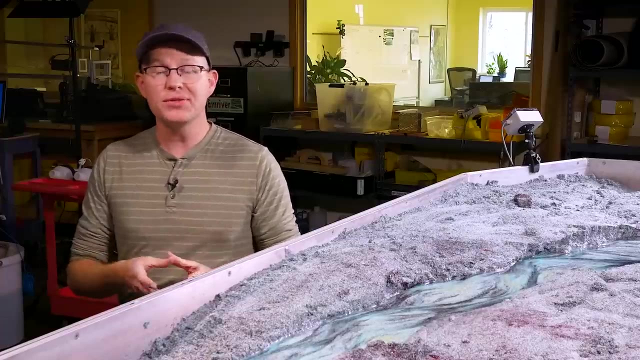 is mostly sediment-free, giving it more capability to cause erosion to the channel downstream. But there's a third impact, maybe more important than the other two. that happens well away from the reservoir itself. Can you guess what it is? In the previous video of this series, we talked about the framework that engineers 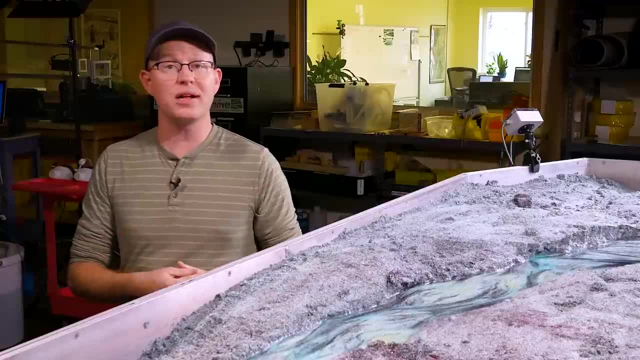 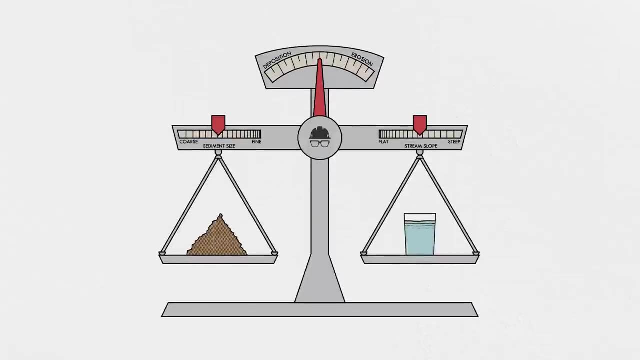 and the scientists who study rivers, called fluvial geomorphologists, use to understand the relationship between the flow of water and sediment in rivers. This diagram, called Lane's Balance, simplifies the behavior of rivers into four parameters: Sediment volume, sediment size, channel flow and channel slope. 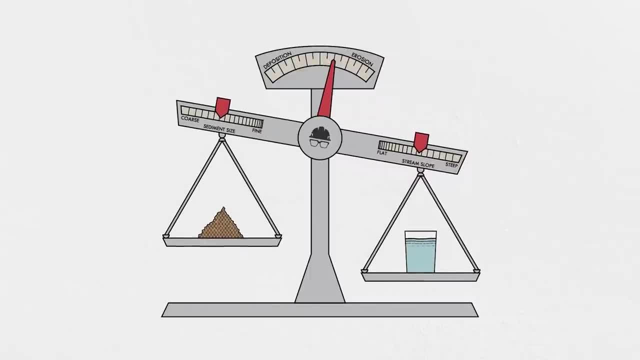 You can see, when we reduce the volume of sediment in a stream, like we would by building a dam, Lane's Balance tips out of equilibrium into an erosive condition. In fact, according to Lane's Balance, anytime we change any of these four factors, it has a consequence on the rest of 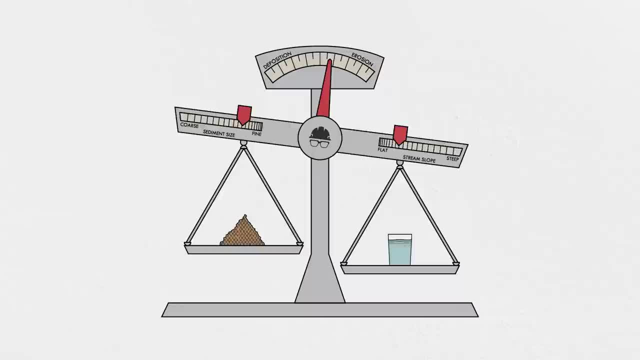 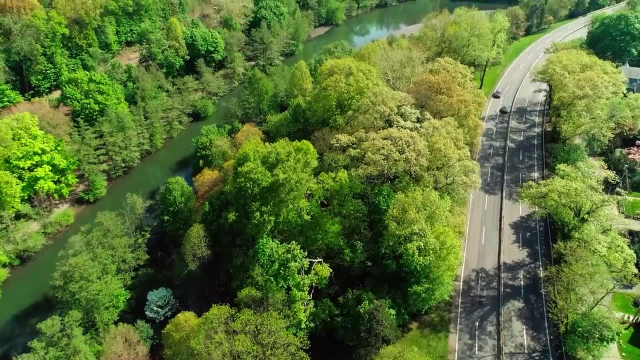 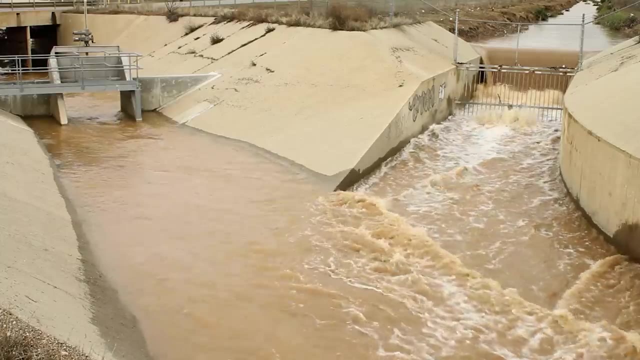 the river as the other three factors adjust to bring the stream back into equilibrium. through erosion or deposition of sediments make a lot of changes to rivers. We want them to stay in one place to allow for transportation and avoid encroaching on property. We want them to drain efficiently so we don't get floods. 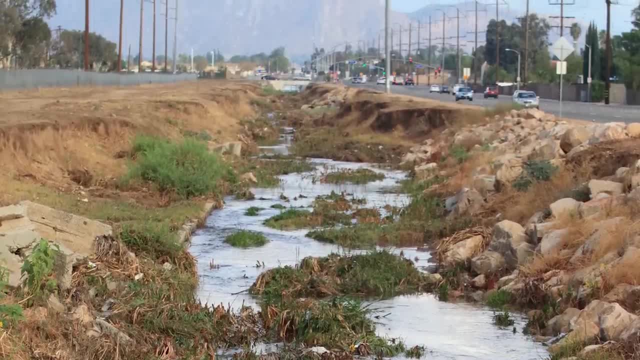 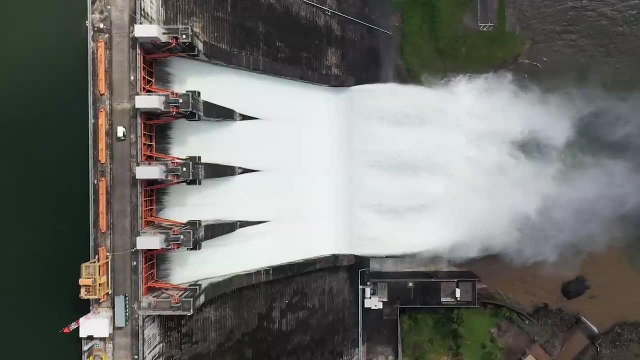 We want them to be straight so that the land on either side has a clean border. We want to cross over them with embankments, utilities, electrical lines and bridges. We want to use them for power and for water supply. Oh, and rivers and streams also serve. 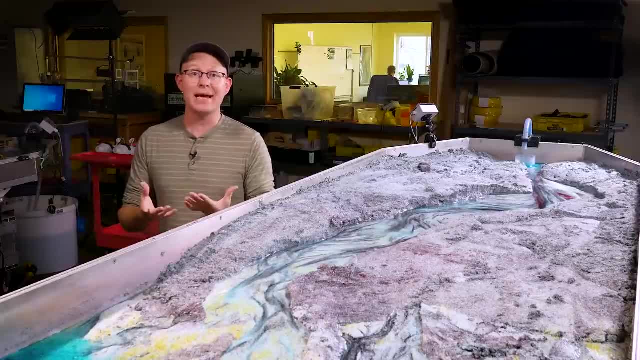 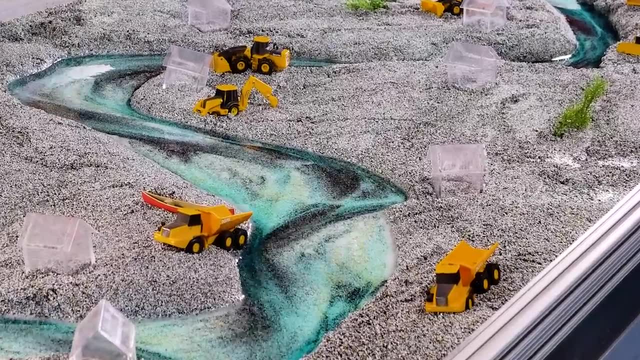 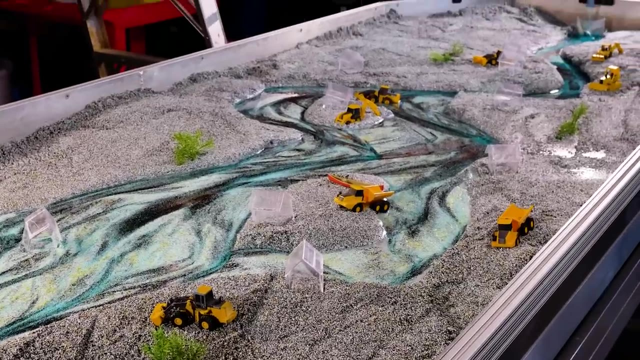 as critical habitat for wildlife that we both depend on and want to preserve. All those goals are important and worthwhile but, as we'll see with the help of this awesome demonstration that can simulate river responses, they often come at a cost, And sometimes that cost is borne by someone. 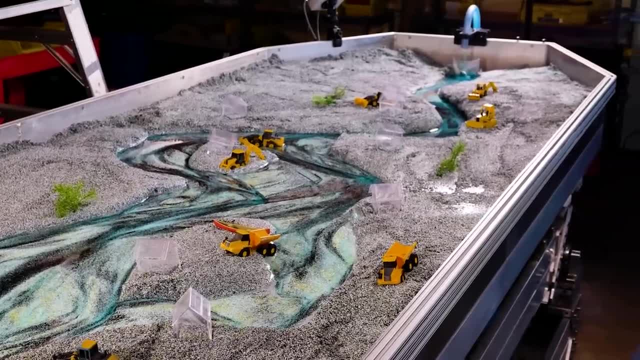 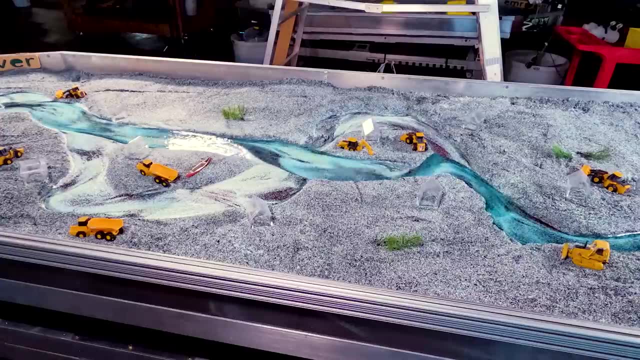 or some place much further upstream or downstream than from where the changes actually take place. One of the classic examples of this is channel straightening. In cities, we often disentangle the river from the stream. We want to make sure that the river is straightened. 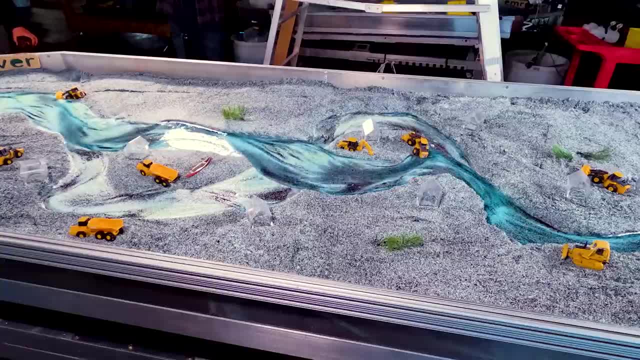 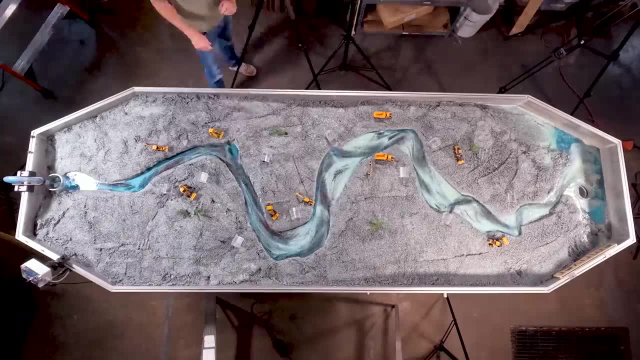 to get water out faster, reduce the impacts of floods and force the curvy lines of natural rivers to be neater so that we can make better use of valuable space. I can show it in the stream table: by cutting a straight line that bypasses the river's natural meanders, The impact of 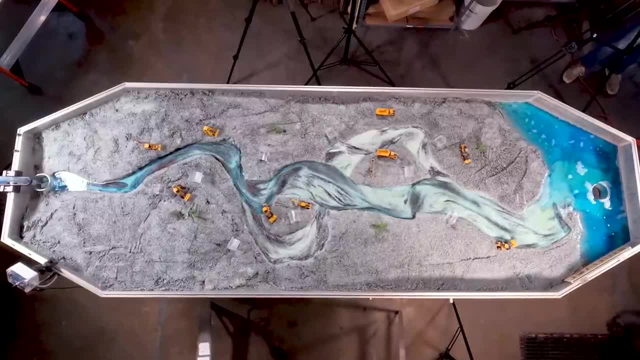 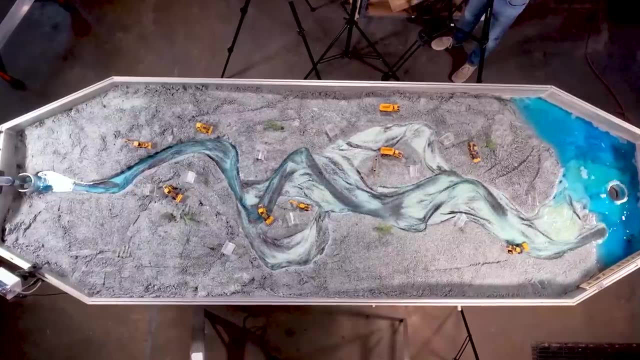 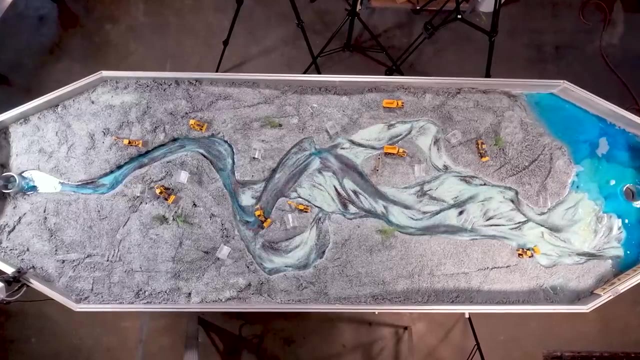 straightening a river is a reduction in the channel's length, necessarily creating an increase in its slope. Water flows faster in a steeper channel, making it more erosive, so the practical result of straightening a channel is that it scours and cuts down over time. It's easy to see the results in the model. This is compounded by the fact that cities have lots of impermeable surfaces that send greater volumes of runoff into streams and rivers. That's why you often see channels covered in concrete in urban areas to protect against the erosion brought on by faster flows. 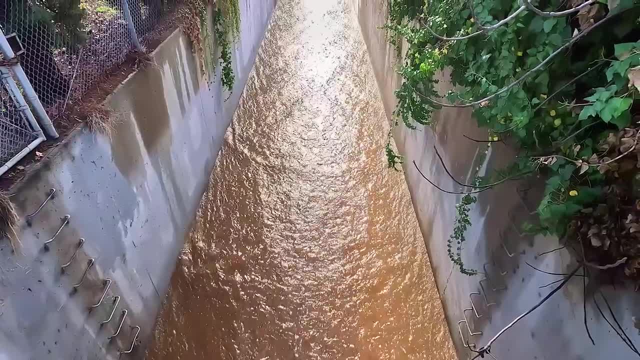 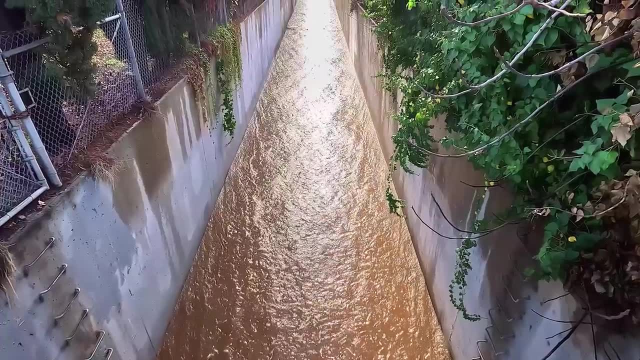 And this works in the short term. but making channels straight, steep and concrete-covered ruins the stream or river as a habitat for fish, amphibians, birds, mammals and plants. It also has the potential to exacerbate flooding downstream because, instead of floodwaters being 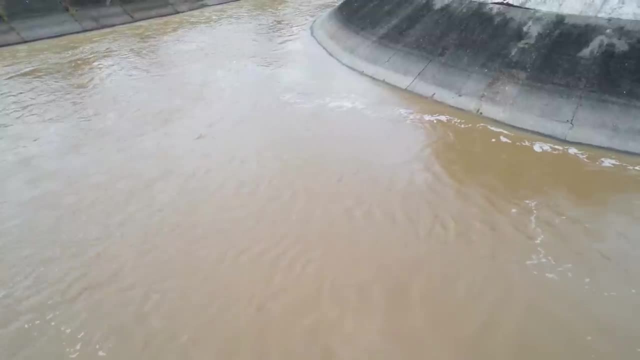 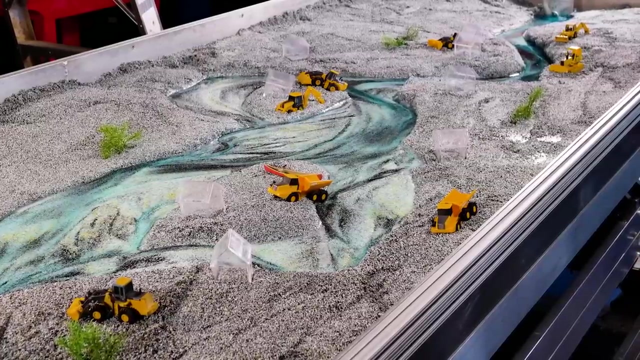 stored and released slowly from the floodplain, it all comes rushing as a torrent at once. instead, And it's not just cities, Channels are straightened in rural areas too, to reduce flooding impacts to crops and make fields more contiguous and easy to farm. 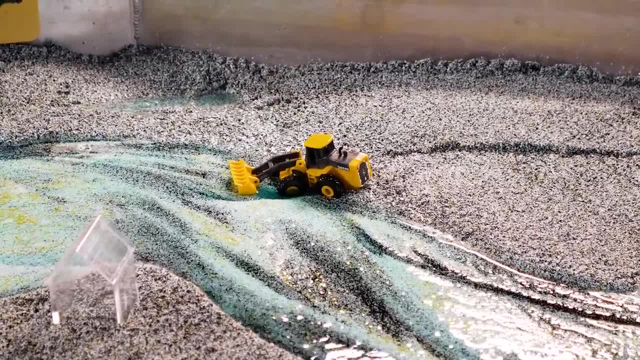 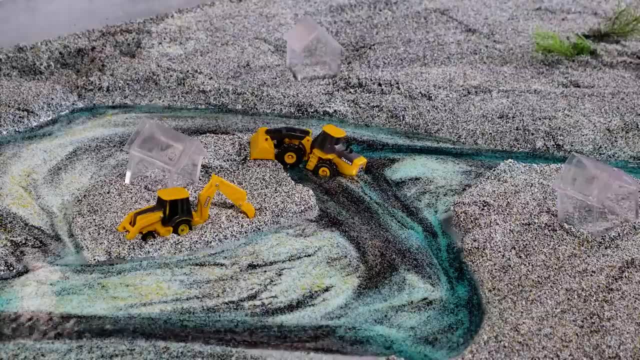 But over the long term. channelizing streams reduces the influx of nutrients to the soils in the floodplain by reducing the frequency of a stream coming out of its banks, slowly making the farmland less productive. Stream restoration is big business right now, as we've begun to recognize these long-term. 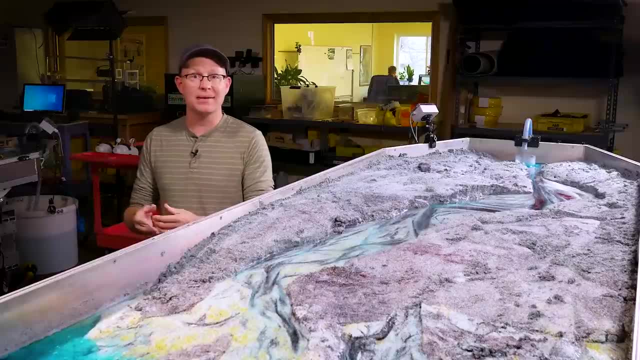 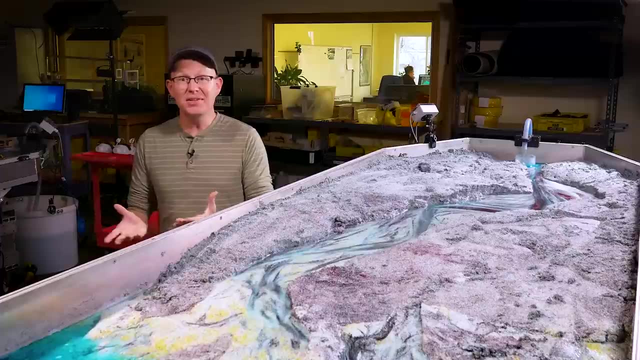 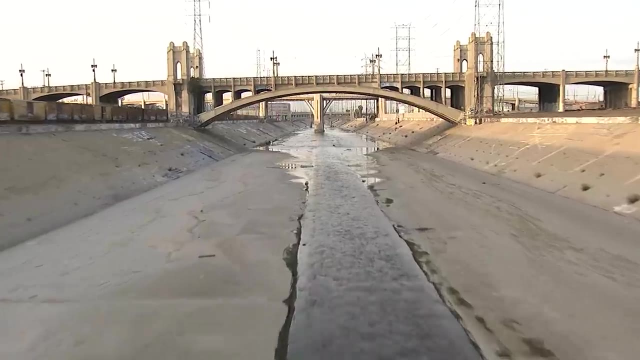 impacts that straightening and deepening natural channels have. In the United States alone, communities and governments spend billions of dollars per year undoing the damage that channelization projects have caused. Even the most famous of the concrete channels, the Los Angeles River, is in the process of. 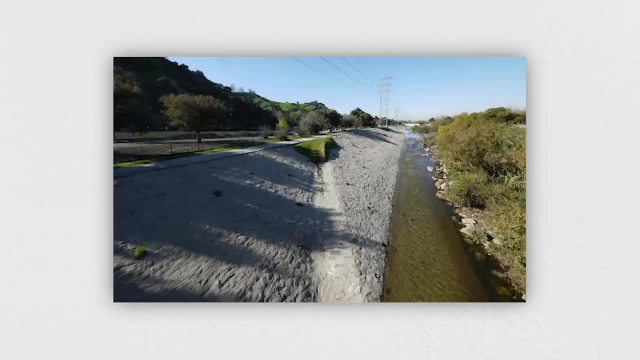 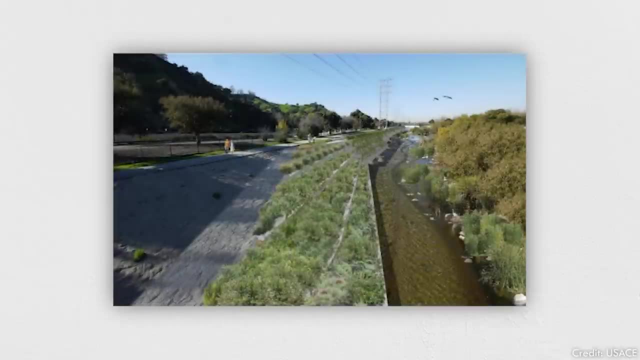 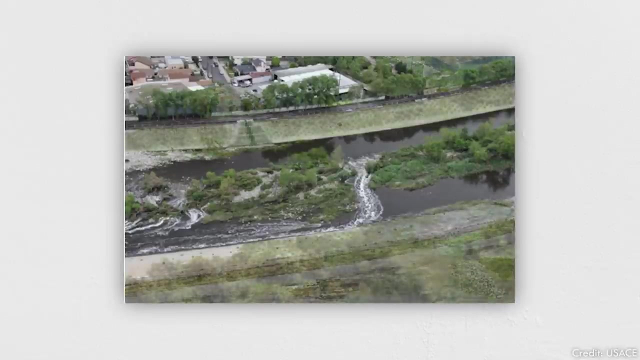 being restored to something more like its original state. The LA River Ecosystem Restoration Project plans to improve 11 miles or 18 kilometers of the well-known Concrete Behemoth in popular films like Grease and Dark Knight Rises. The project will involve removing concrete structures to establish a soft bottom channel. 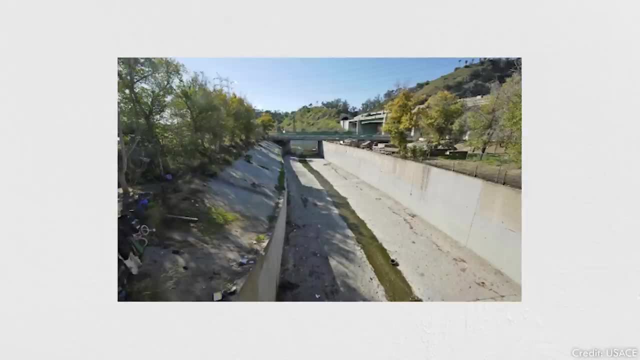 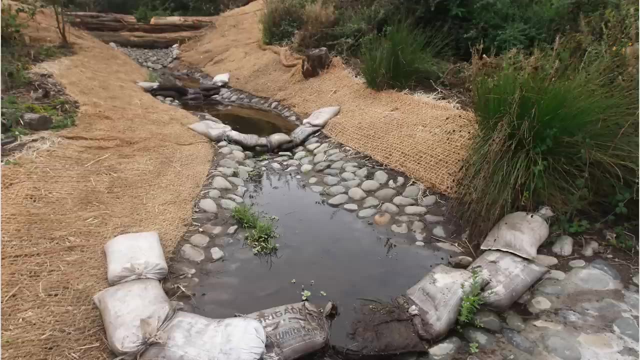 daylighting streams that currently run in underground culverts, terracing banks with native plants and restoring the floodplain areas, giving the river space to overbank during floods, Thanks to fluvial geomorphologists. projects like this are happening all around the world. 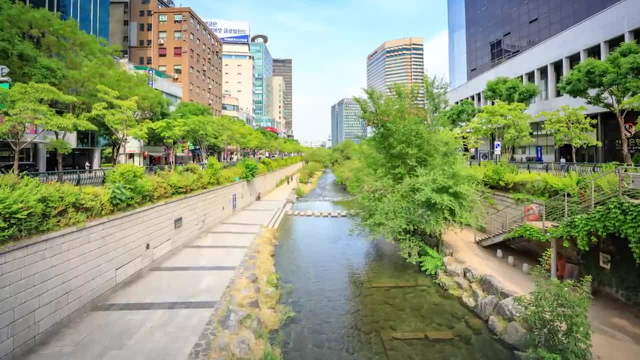 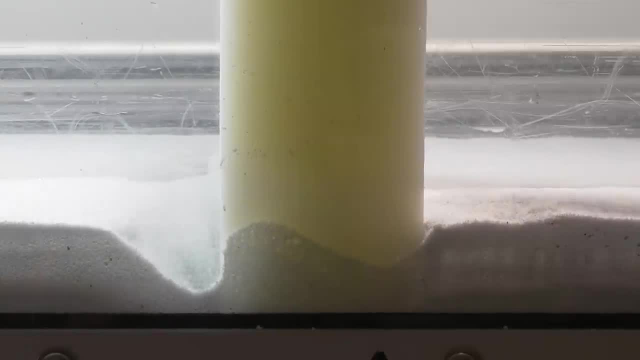 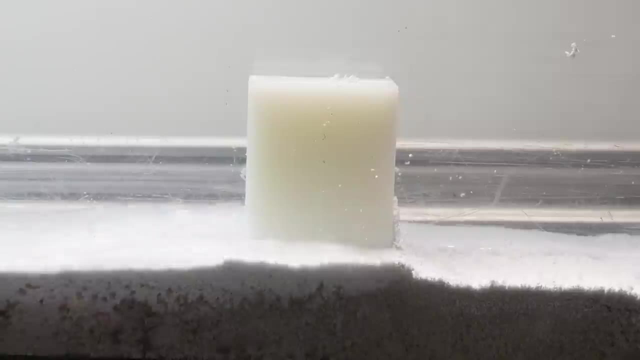 But straightening channels isn't the only way humans impact rivers and streams. Another impactful place is at road crossings. Bridges are often supported on intermediate piers or columns that extend up from a foundation in the riverbed. Water flows faster around the obstruction created by these piers, making them susceptible. 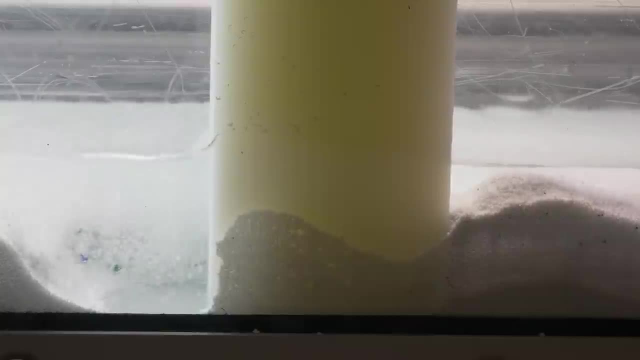 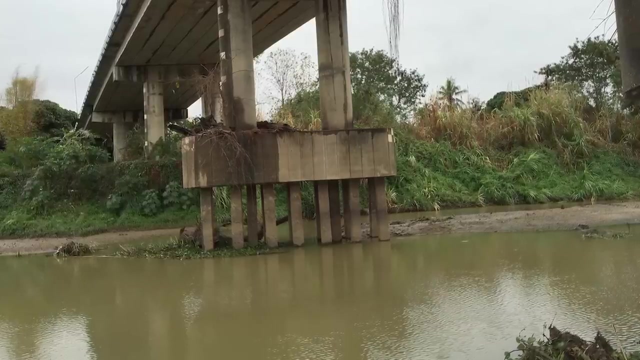 to erosion, and scouring Engineers have to estimate the magnitude of the scour to make sure the piers can handle it. You don't have to scour the internet very hard to find examples where bridges met their demise because of the erosion that they brought on themselves. 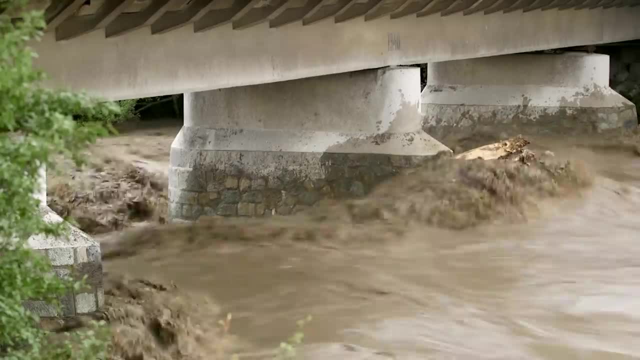 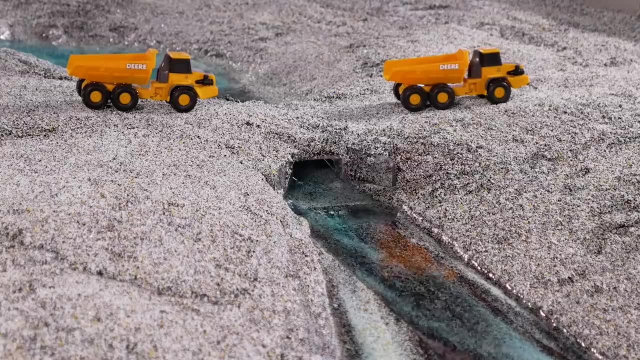 In fact, the majority of bridges that fail in the United States don't collapse from structural problems or deterioration. They fail from scour and erosion of the river below. But it's not just piers that create erosion. Both bridges and embankments equipped with culverts often create a constriction in the 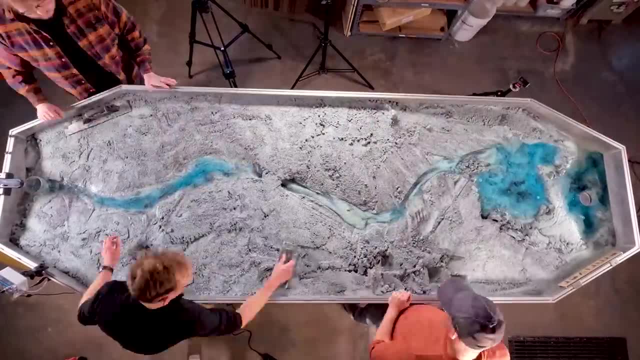 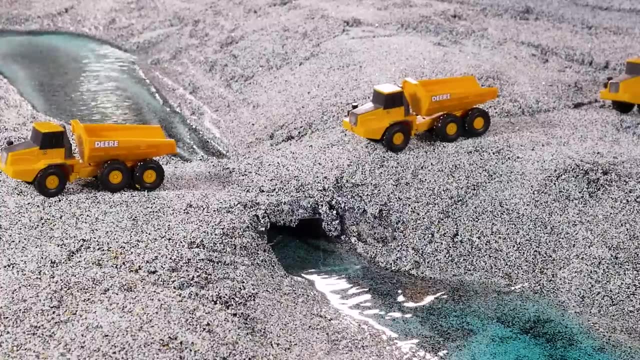 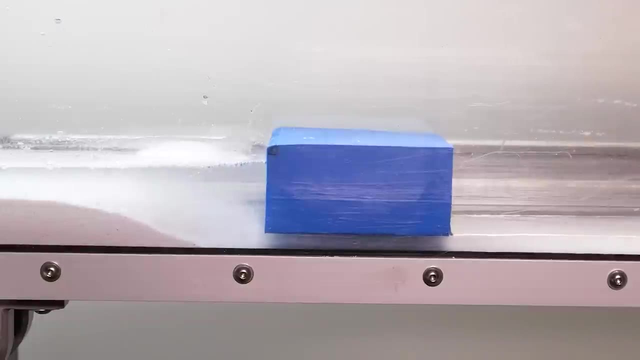 channel as well. Bridge abutments encroach on the channel, reducing the area through which water can flow, especially during a flood, causing it to contract on the upstream side and expand on the downstream side. Changes in the velocity of water flow lead to changes in how much sediment it can carry. 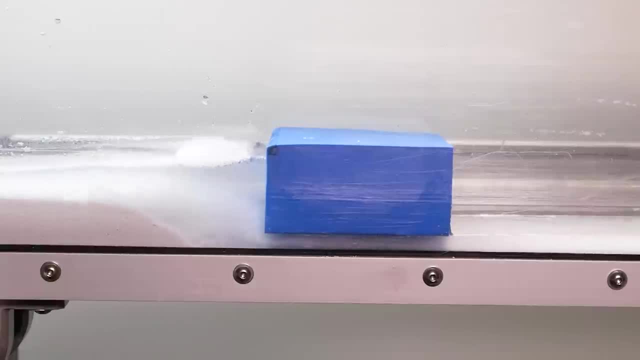 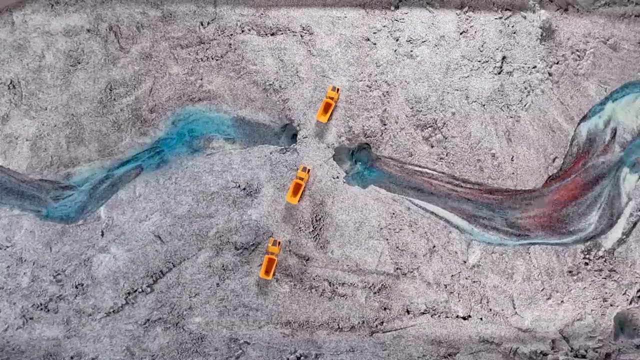 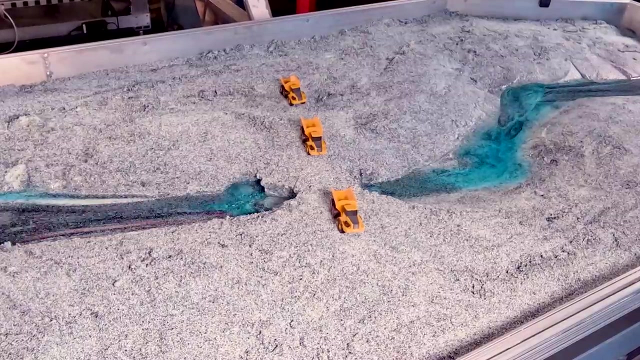 Often you'll see impacts on both sides of an improperly designed bridge or culvert. Sediment accumulates on the upstream side, just like for a dam, and the area downstream is eroded and scoured. Modern roadway designs consider the impacts that bridges and culverts might have on the 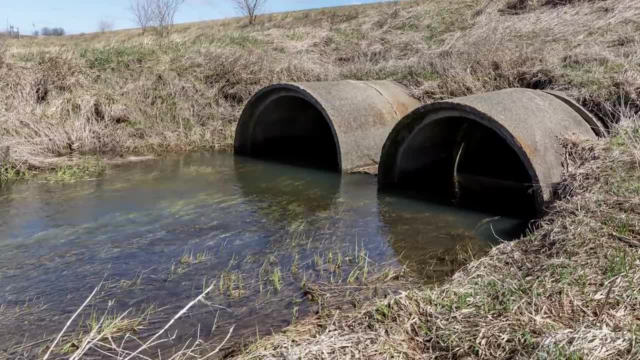 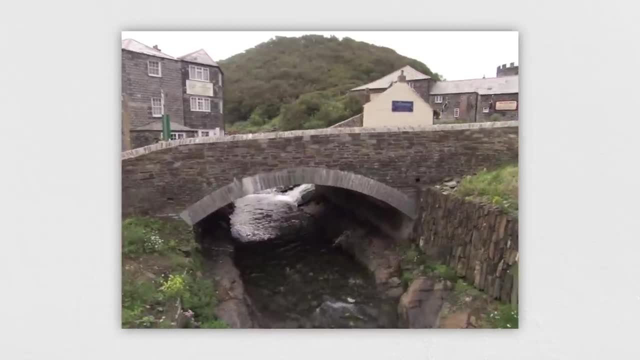 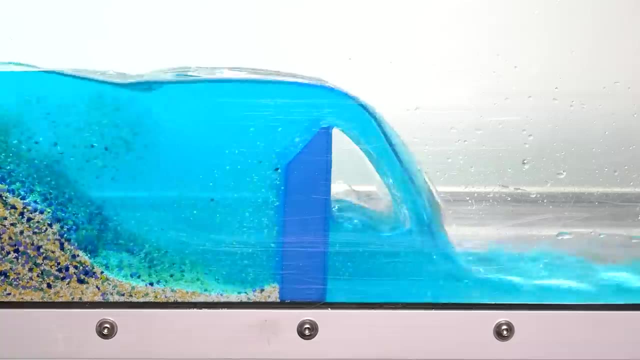 stream to avoid disrupting the equilibrium of the sediment balance and reduce the negative effects on habitat too. Usually that means bridges with wider spans so that the abutments don't intrude into the channel, and culverts that are larger and set further down into the stream bend. 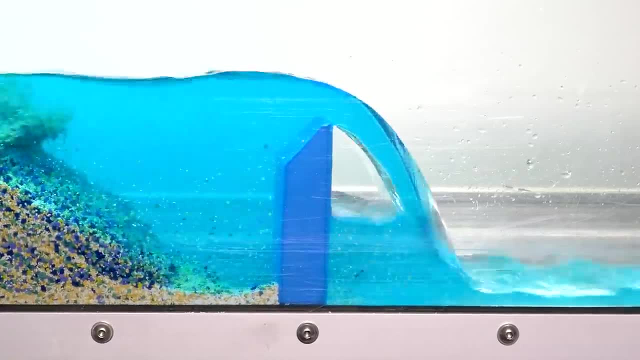 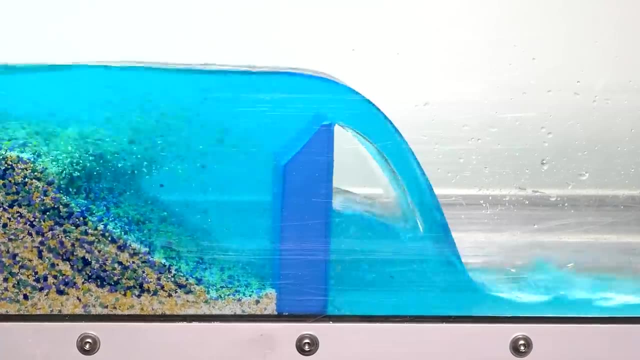 Just like bridges or culvert road crossings, dams slow down the flow of water upstream, allowing sediment to fall out of suspension, as we saw in the flume earlier in the video. The consequences include sediment accumulation. The dams slow down the flow of water upstream, allowing sediment to fall out of suspension, as we saw in the flume earlier in the video. 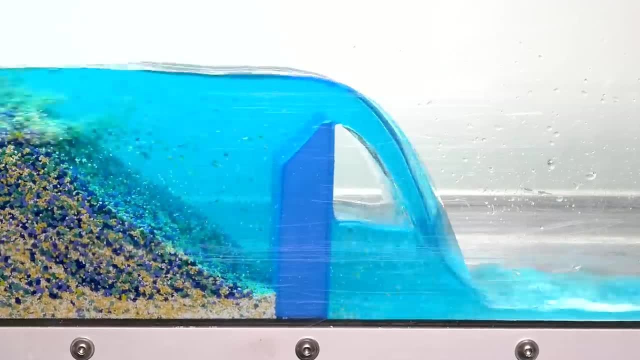 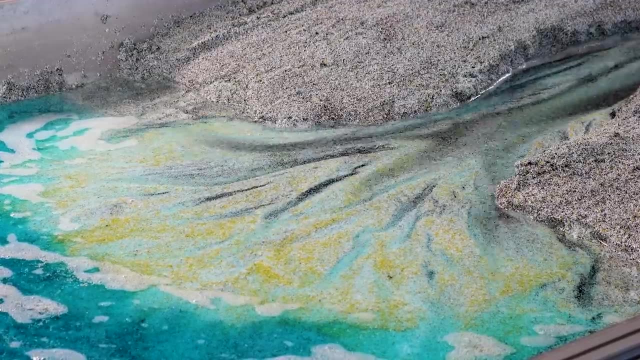 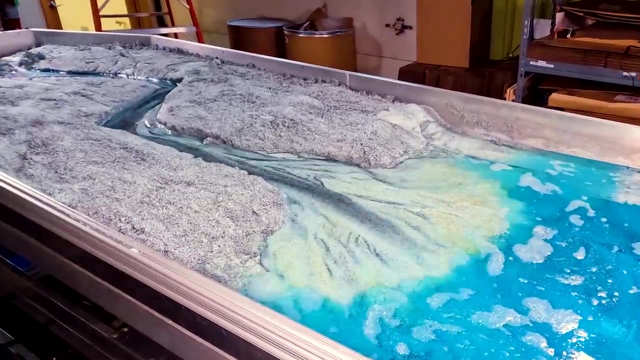 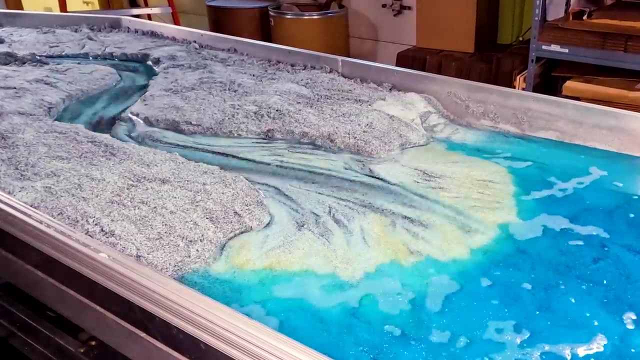 All that silt, sand and gravel that a dam robs from the river has a natural destination: The delta. When a river terminates in an ocean, sea, estuary or lake, it normally deposits all that sediment. Let's watch that process happen in the river table. 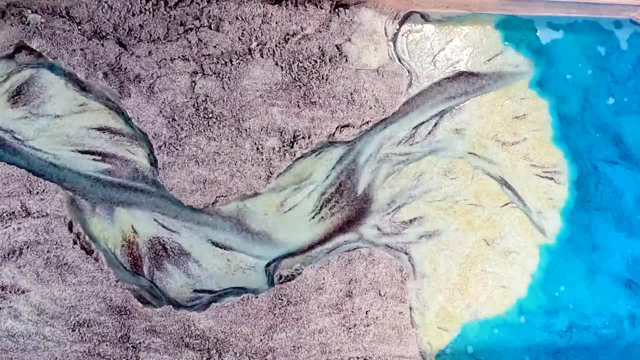 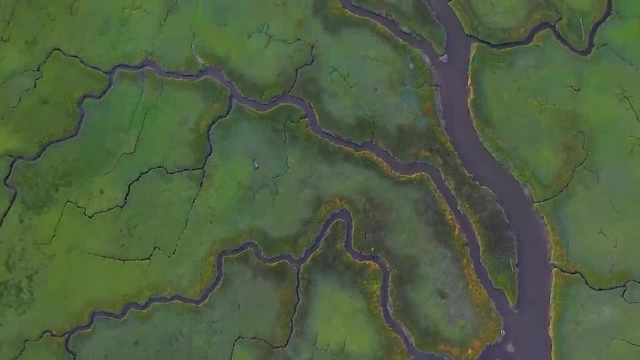 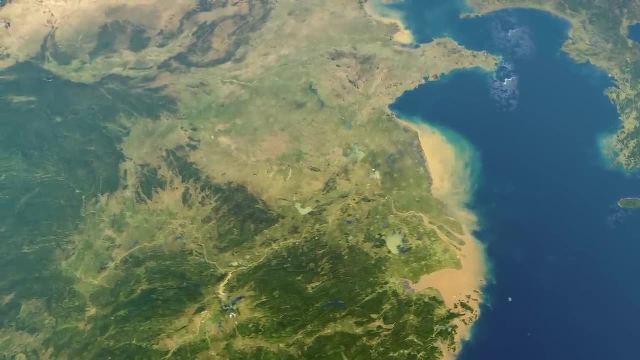 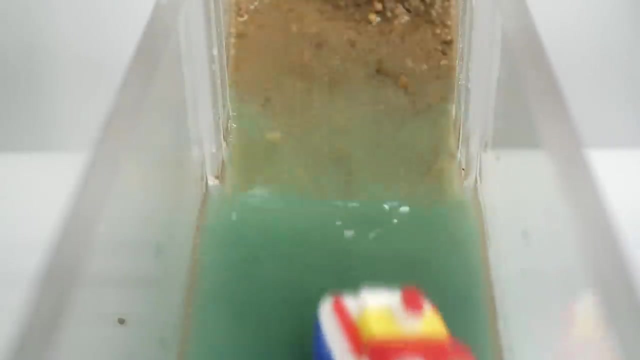 River deltas are incredibly important landscape features because they enable agricultural production, provide habitat for essential species, and they feed the sand engines to create beaches that act as a defensive buffer for coastal areas. Wind and waves create nearly constant erosion along the coastlines, and if that erosion 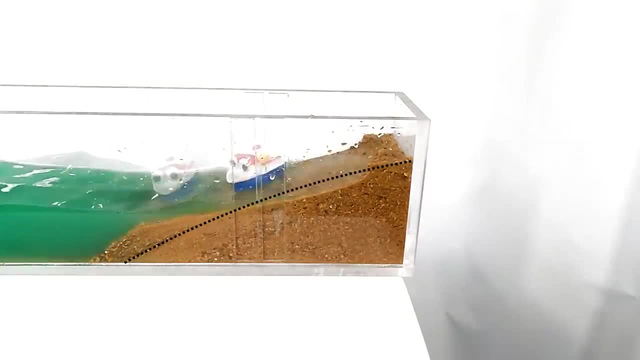 isn't balanced with a steady supply of sediment. beaches scour away, landscapes are claimed by the sea, habitats degraded and coastal areas have less protection against storms. And hopefully you're seeing now why it's so difficult and some might even say impossible. to control rivers, Because any change you make upsets the dynamic equilibrium between water and sediment. And even if you armor the areas subject to erosion and continually dredge out the areas subject to deposition, There's always a bigger flood around the corner, ready to unravel it all over again. 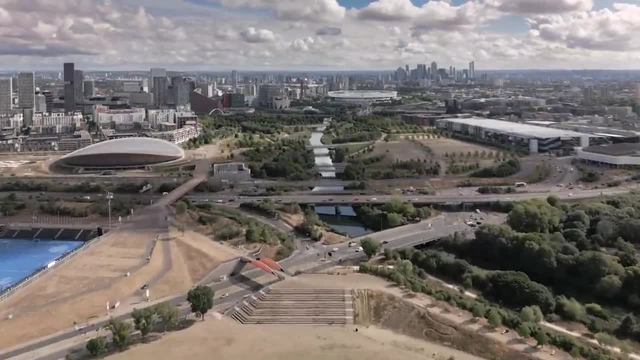 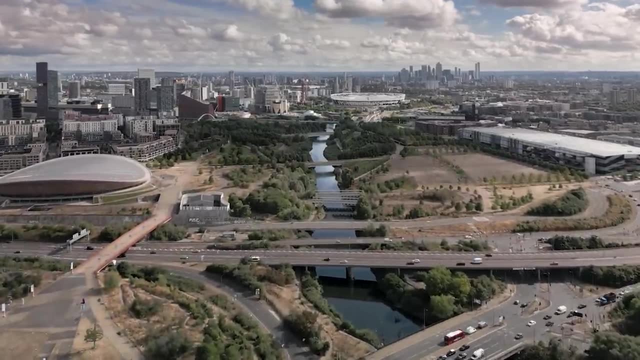 So many human activities disrupt the natural equilibrium of streams and rivers, causing them to either erode or aggrade, or both, And often the impacts extend far upstream or downstream. It's not just dams, bridges and channel realignment projects either. 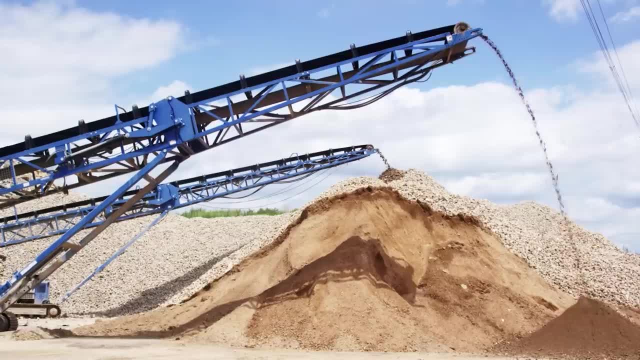 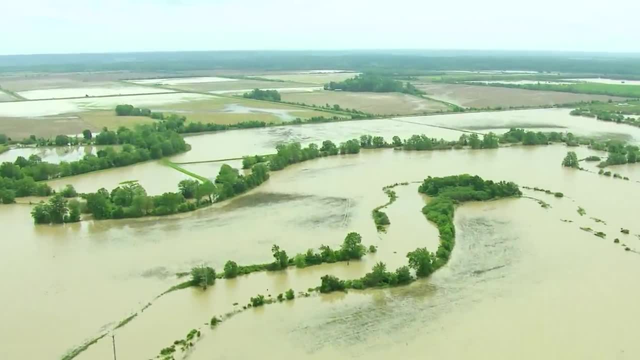 We build levees and revetments, dredge channels, deeper mine gravel from banks, clear-cut watersheds and more. Historically, we haven't fully grasped that. We haven't grasped the impact that those activities will have on the river in 10, 50,. 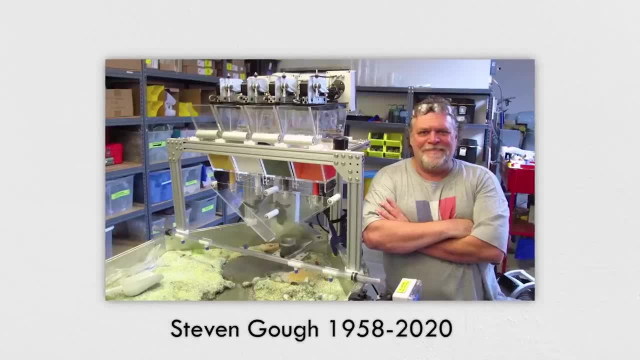 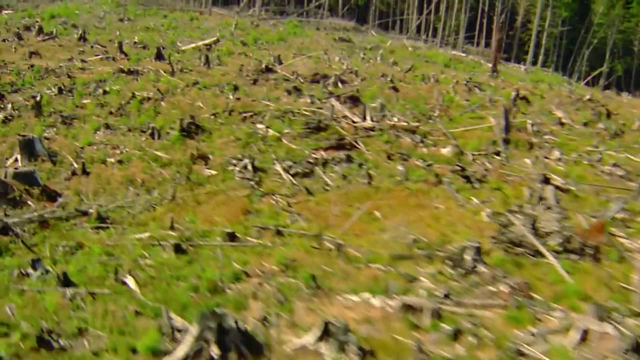 or 100 years. In fact, the first iteration of the stream tables we've been filming were built by Imrivers' late founder Steve Goff in the 1980s. At the time he was working with the state of Missouri trying to teach miners loggers. 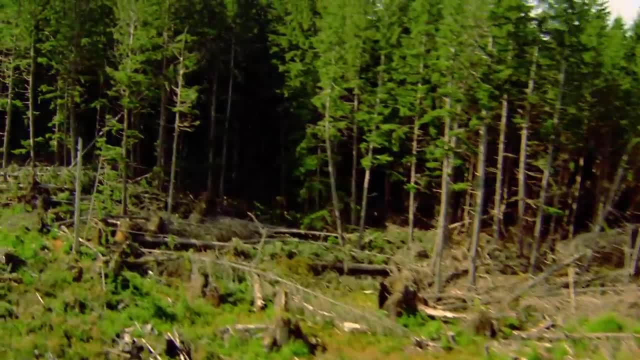 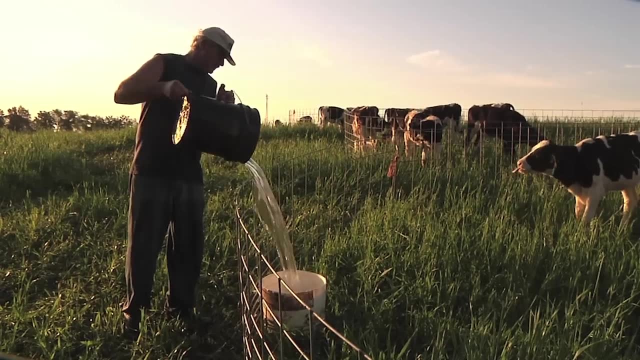 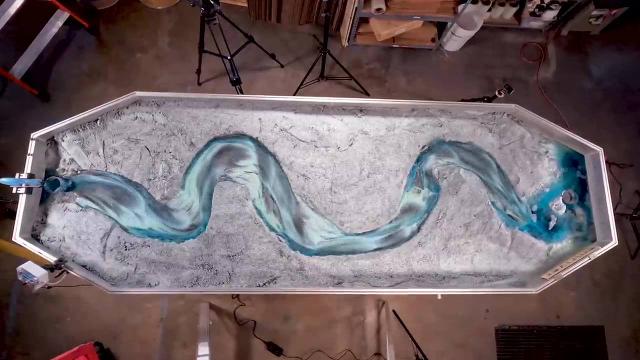 and farmers about the impacts they could have on rivers by removing sediment or straightening channels. These people, who had observed the behavior of rivers their entire lives, were understandably reluctant to accept new ideas. But seeing a model that could convey the complicated processes and responses of rivers, 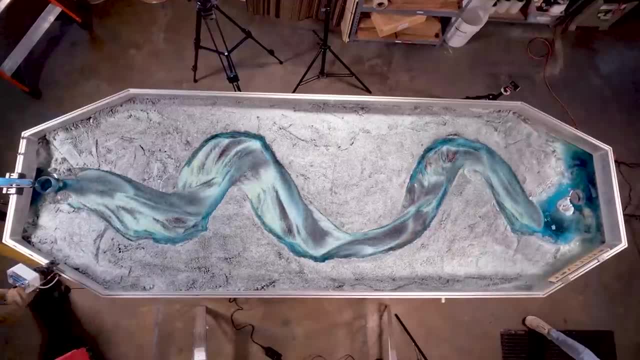 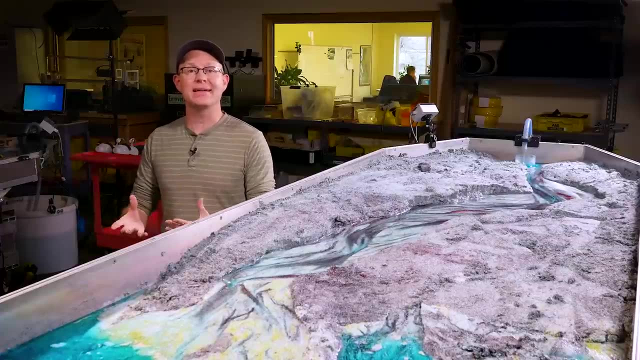 was often enough to convince those landowners to be better stewards of the environment. Huge thanks to Steve's wife, Katherine, and the whole team here at Imriver, who continue his incredible legacy of using physical models to shrink down the enormous scale of river. 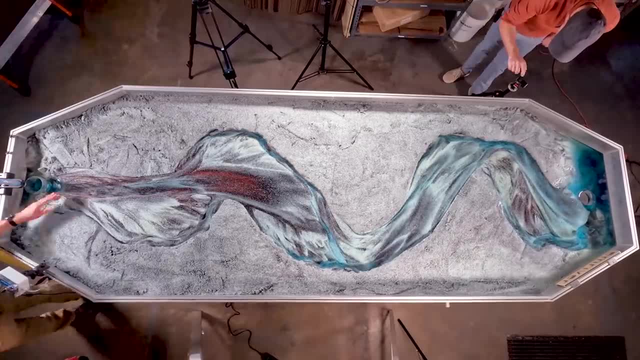 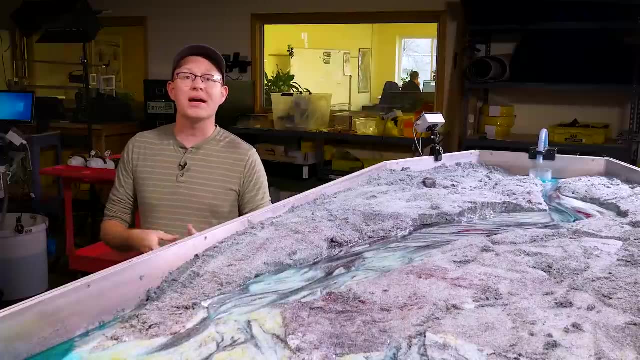 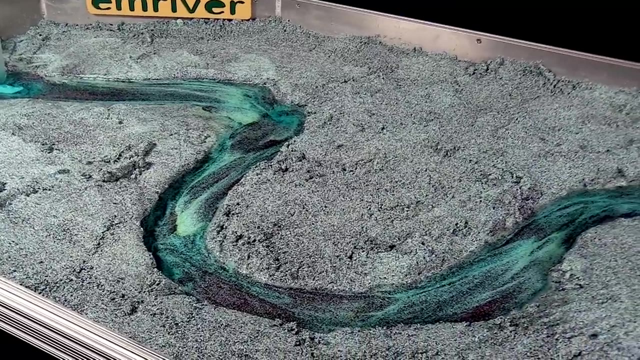 systems and the lengthy timescales over which they respond to changes, down to something anyone can understand, to help people around the world learn more about the impacts of the confluence of engineering and natural systems. Historically, engineering and fluvial geomorphology have been entirely separate fields of study. 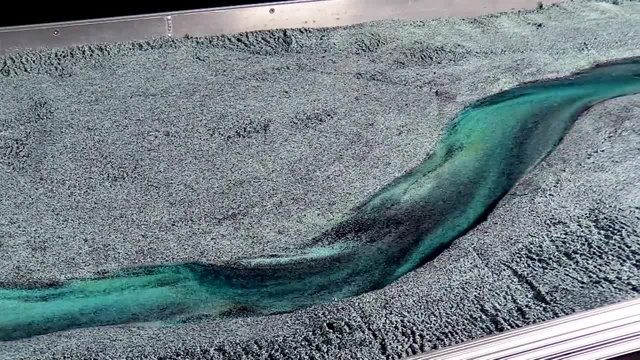 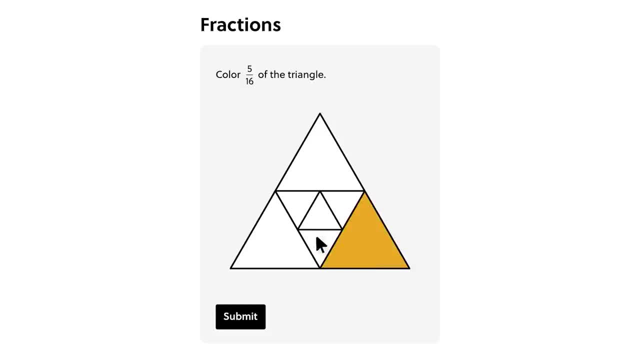 Which means if you were an engineer and wanted to learn more about the impacts engineering projects have on natural streams, you had to do some extracurricular learning. If you've done it, you know teaching yourself math and science is a hard thing to do. 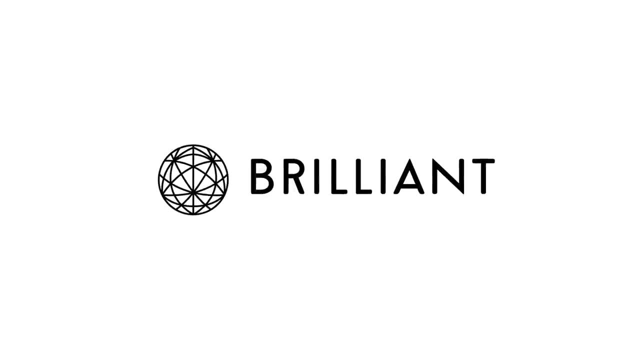 A problem that today's sponsor, Brilliant dot org, takes on head first. There are more things you can learn about natural systems than you can do about them, which are not the same as the fact that there is no plus and minus to learning a natural system. 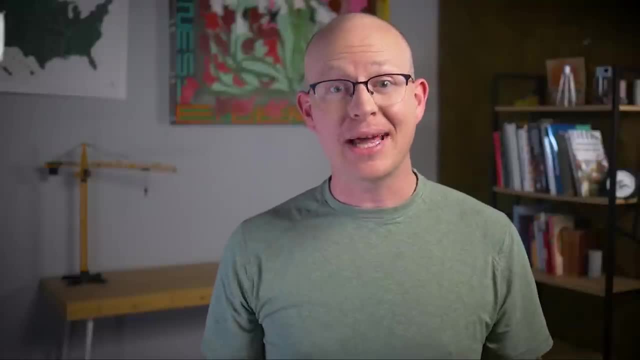 There's so much to learn about the natural systems that you won't have to feel like things you learn in school that you don't end up needing in life. But if you're like me, there are just as many things you didn't learn in school that you need to know now to get ahead in your 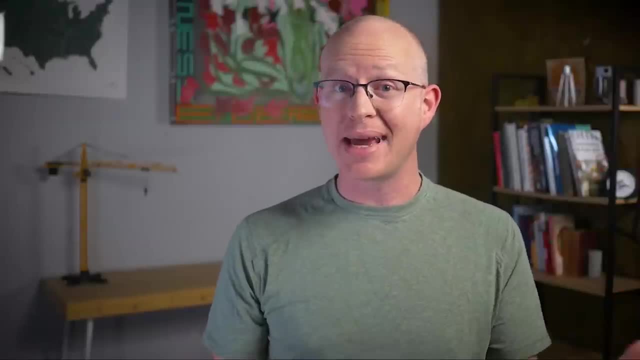 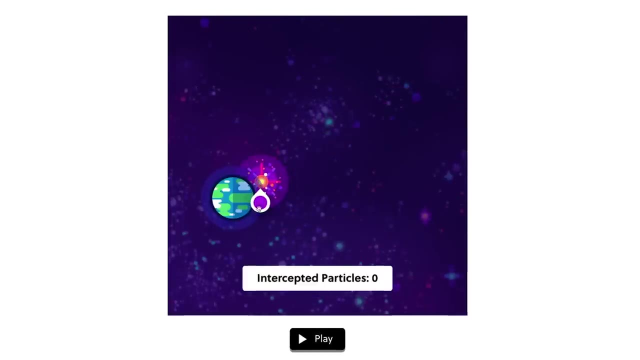 career, reach your personal goals, or just out of pure curiosity and the delight of learning something new. Brilliant is a platform where you learn by doing, with thousands of lessons from math to AI, data science and engineering. I've gone through a lot of these courses to freshen. 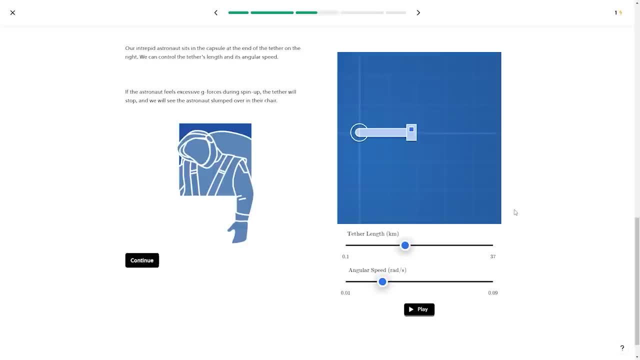 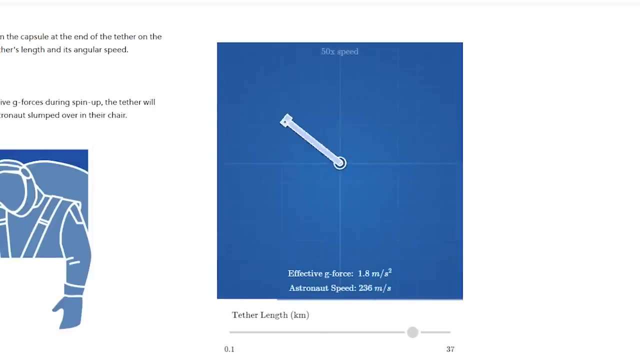 up on topics that are new to me, but my absolute favorite was this one on the physics of rockets and tether launchers by my friend Brian at Real Engineering. It's fun to hear about the engineering challenges of structures like this, but it's a different experience entirely to work. 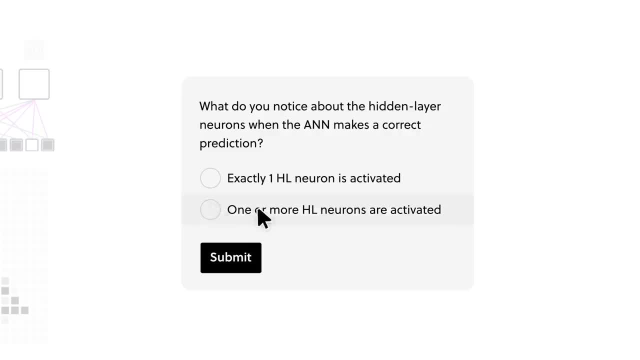 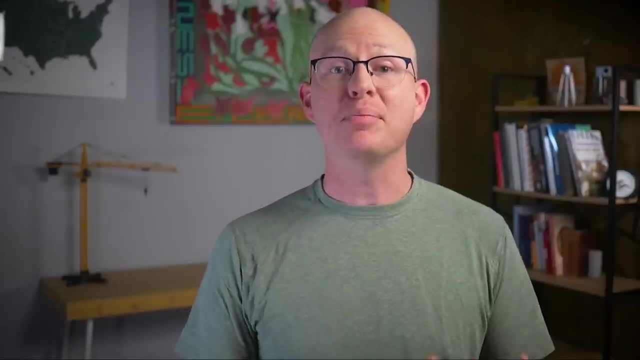 through them yourself. It just gives you a new appreciation for the math and science and a feeling that you really understand the problems in a deep way. You should go try it yourself and see if you agree at brilliantorg slash practical engineering. It's totally free to try for an. 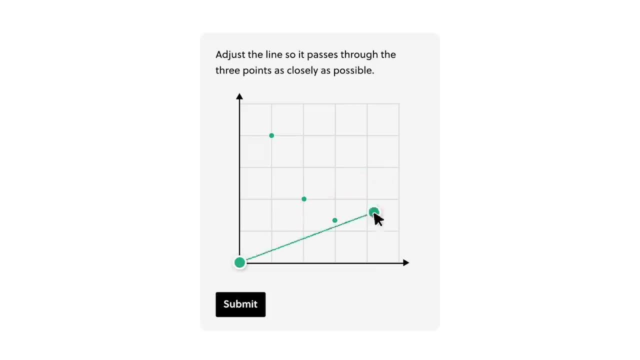 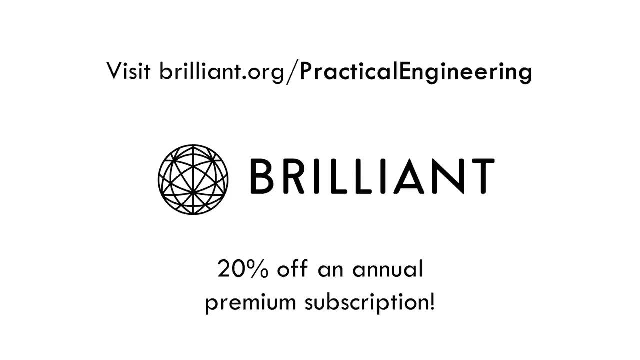 entire month and you could get through a lot of courses in that time. But if you do find yourself coming back to this platform, I'd love to hear from you. I'd love to hear from you. In fact, like I did, the first 500 people that click the link below will get 20% off an annual. 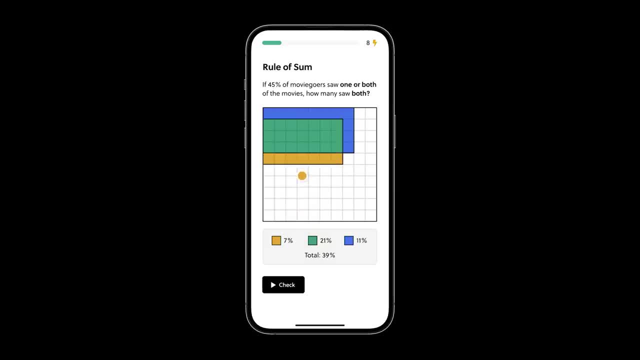 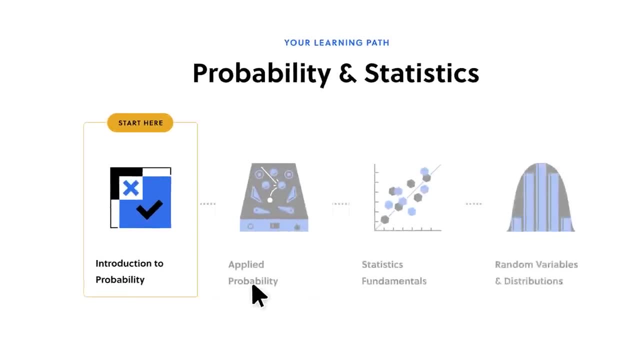 premium subscription. They even have an app so you can try this on your phone. I really believe that we should never stop trying to learn new things, and Brilliant makes that so easy to do, And it supports the channel too. Thank you for watching and let me know what you think. 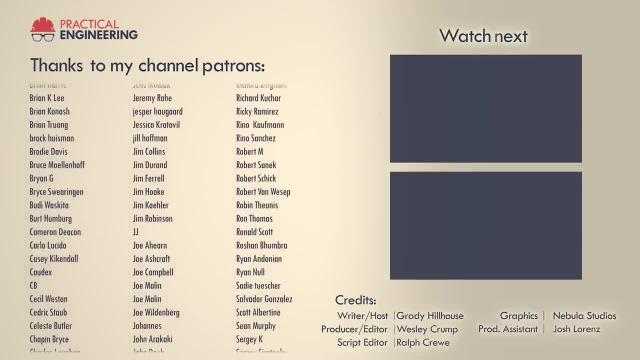 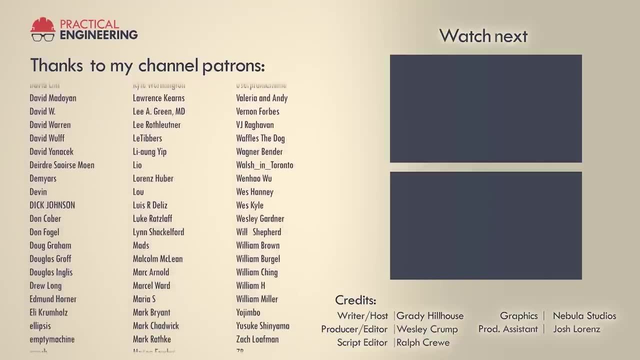 Thank you for watching and let me know what you think.